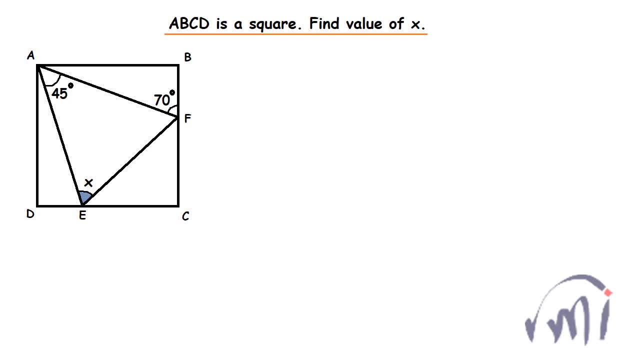 Hi. so here we have a problem which was sent by one of my viewers, and in this problem, a, b, c, d is a square and we have to find the value of x. So a, b, c, d is a square and here we have a 45 degree angle, and here we have a 70 degree angle and we have to find the value of x. So how do we do it? See, if this is 70 degrees, then this will be equal to 20 degrees, because this is 90 degrees and this angle is 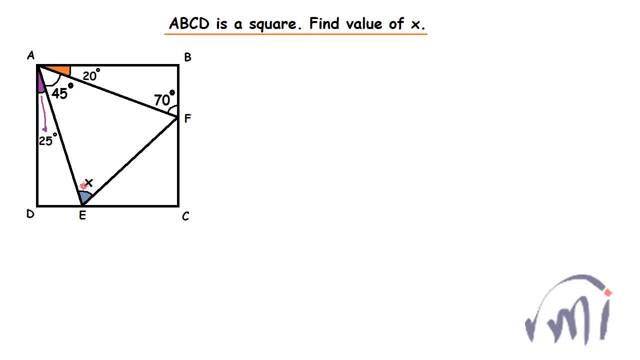 will be equal to 25 degrees, and we have to find the value of this angle, which is denoted as x, and for this I'll make another copy of this over here and now. what I'm going to do is I'm going to copy this triangle a, b, f and paste it over here. Then let me remove all this and it will look something like this. and here: if this angle was 25 degrees, that means this angle would have been 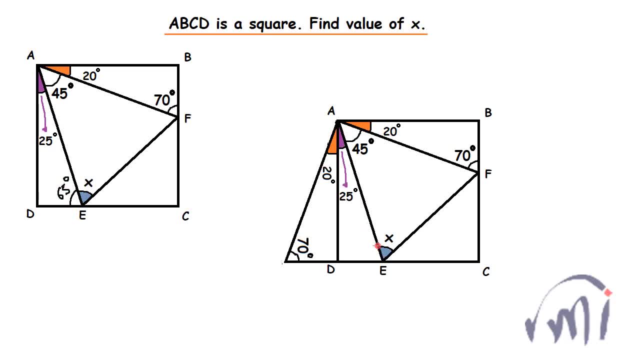 60 degrees, Right. So this angle is actually 65 degrees and since this triangle a f t is congruent to triangle a f b, that means this is 90 degrees and side a f is actually equal to side a f Right. And if you see properly, this side a e is actually present in both the triangles: triangle a f e and triangle a f e. 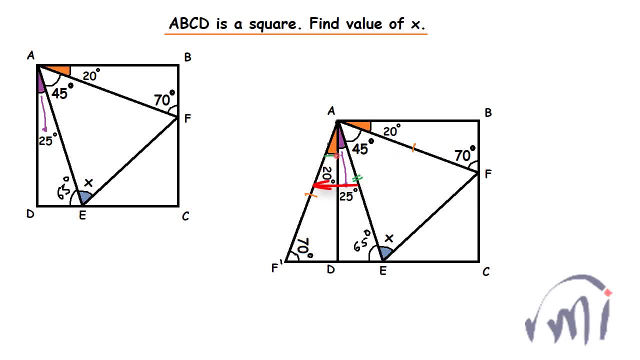 So these two sides are equal and if I talk about this total angle, this angle is actually equal to 20 plus 25, 45, and this angle, angle f- a- e, is also equal to 45. That means triangle a- f- e and triangle a- f- t. both of them are congruent. That means the corresponding angles- angle a- e- f' and angle a- f- e- are congruent. 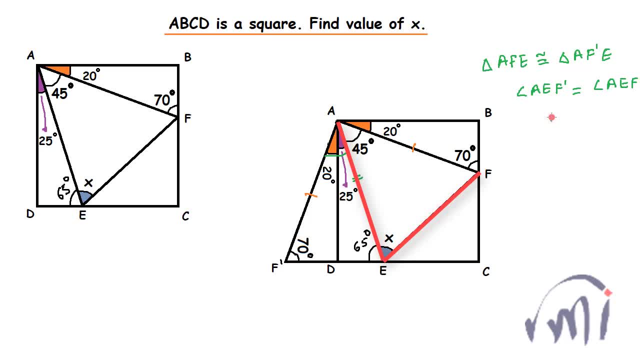 AEF, both of them will be equal and both of them will actually be equal to 65 degrees, right? So the value of x is actually equal to 65 degrees. So that's all for this video, and if you also have an interesting problem for which you need a solution,